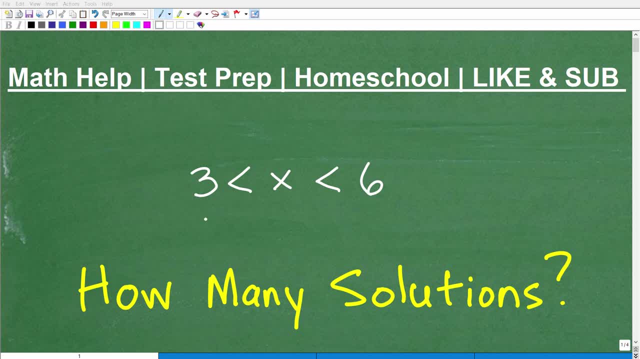 Okay, so let's talk about basic algebra, just basic mathematics. So this is what we call an inequality, And hopefully you're looking at this and you can understand these symbols right here. You've seen these. This has to do with- I'm going to kind of give you a little bit of a hint- less than, greater than, less than, or equal to, greater than or equal to, etc. So this is the topic of inequalities, And we have this specific inequality right here And I'm asking you: how many solutions do you have? 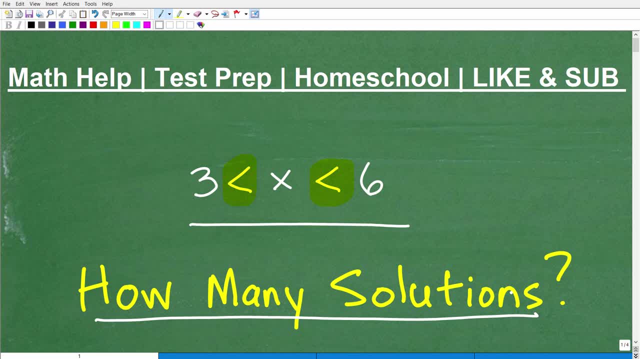 Does this inequality have? So I'm going to kind of purposely be vague about it right now because I want you to think about it, But if you know the answer, go to put that into the comment section. Of course, I'm going to cover this in detail in just one second, But first let me quickly introduce myself. My name is John. I'm the founder of TC Math Academy. I'm also a middle and high school math teacher. I've been teaching math for decades And I'm telling you right now, if you're struggling in math, there is hope. Okay, you could do much, much better than you currently are, So don't give. 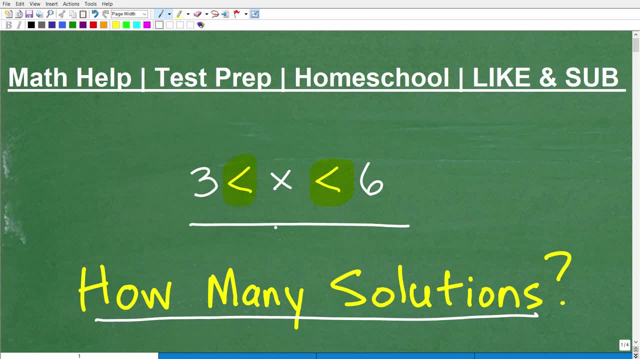 up. Basically, to do well in math requires two things. One, you got to have a strong work ethic. you got to be willing to work hard. So that's the first thing. The second thing is you need great math instruction- clear, understandable, comprehensive, And that's where I can help you out. So if you're at the middle school, high school or college level, check out my math help program. You can find a link to it in the description of this video. Also, if you happen to be studying for a particular test that has a math section on it, a dedicated math section, things like the GED. 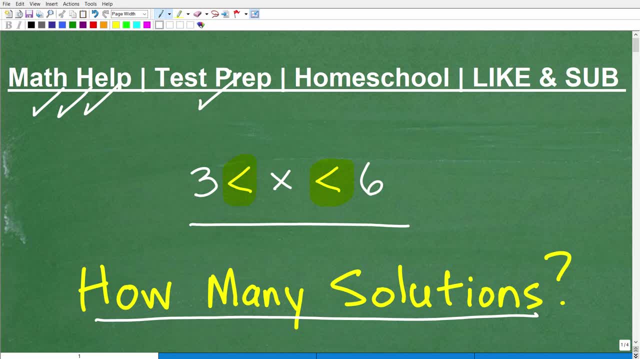 SAT, ASVAB, maybe a teacher certification exam. I have a ton of test prep courses that can help you out. If you're homeschooled, definitely check out my middle and high school math programs for homeschoolers. They get excellent reviews. And then also, if this video helps you out, don't 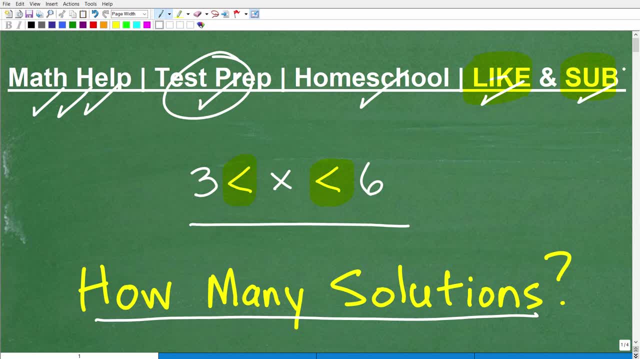 forget to help me out by liking it and subscribing to my channel. Okay, so let's get into this problem. How many solutions does this inequality have? Well, first of all, let's kind of interpret what's this inequality is saying. So what symbol is this? Okay, is this the greater than or less? 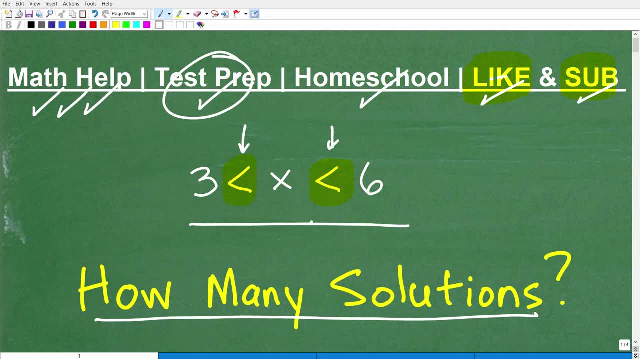 than Okay. so this symbol, it happens to be this symbol right here. Well, the way to remember the difference is, if you notice this symbol kind of looks like a kind of sideways L. So this is the less than Okay. so this is the best way to kind of remember these symbols So you don't confuse. 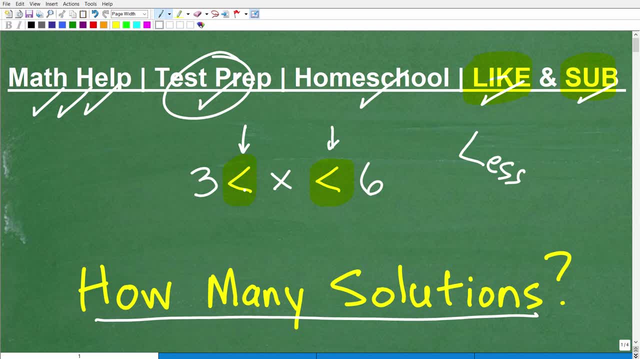 this You're like: is this greater than or less than? Well, the way it's written right here, this is the less than symbol. Okay, so that's the first thing. Then we have this variable x right here in the center, And what is that saying? Well, x represents some number, right? So 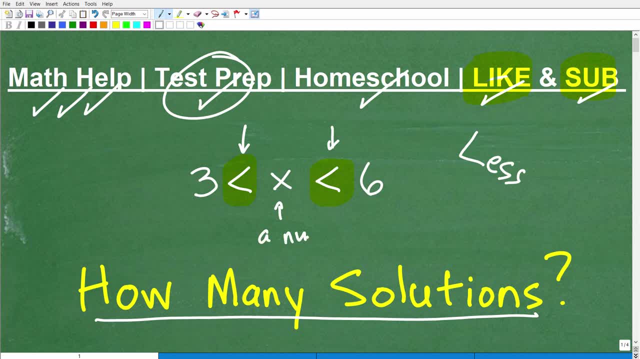 this is going to put in a number, number or numbers. This is important, Okay, not just one number, maybe, but maybe more than one number, a number or numbers. So that's what x represents: some possible value. So what we're saying is: 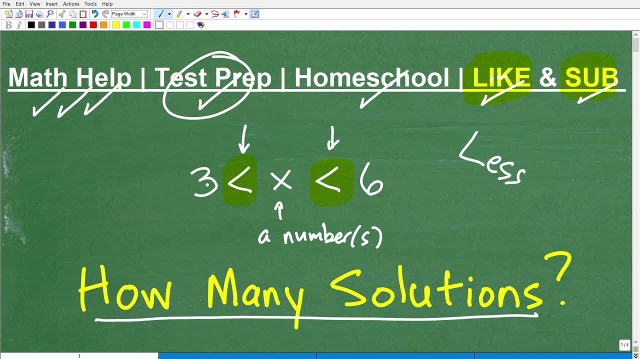 a number or numbers, okay, that are worth three is less than ie this number is greater than three. Okay, so these numbers, all the numbers that are greater than three, okay, ie that this number three is less than whatever number this is. Now, at the same time, we have to look at 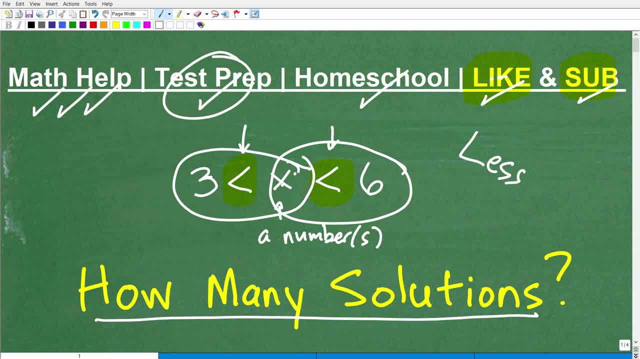 this part of this inequality. So this is saying this number happens to be less than six. So there's kind of two things going on in this. we call this kind of inequality a compound inequality. So just to kind of give you an example of just a basic linear inequality. So if you have x, is this symbol three. this is what. 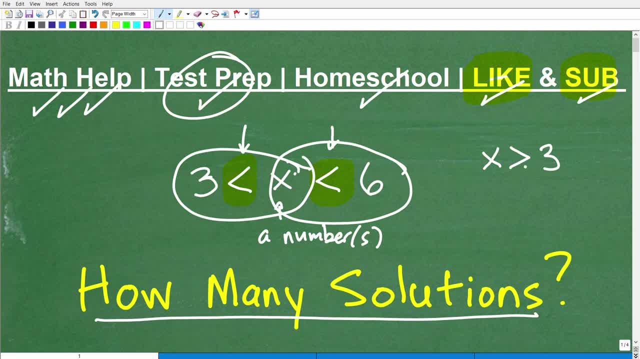 Well, this doesn't look like an L. this is the other one, So this is greater than so. this is x is greater than three, or a number or numbers that are greater than three. Okay, so that's how this right here would be interpreted. So here we have a range of numbers. 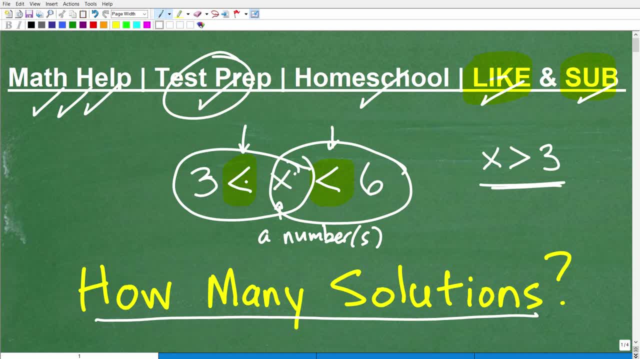 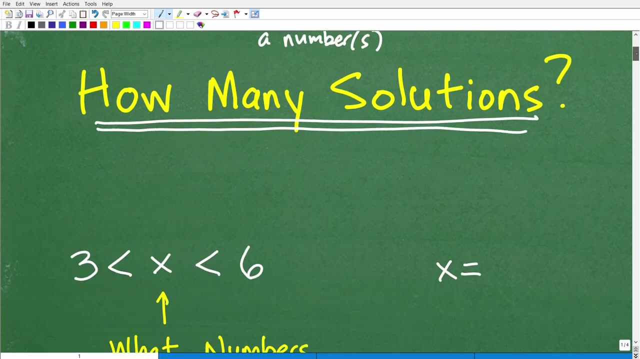 right. So we have numbers that were that are greater than three, and we're looking at it this way- but at the same time less than six. So if that kind of helps, you again go ahead and tell me how many solutions this inequality has. So what does that mean? to have a solution to an 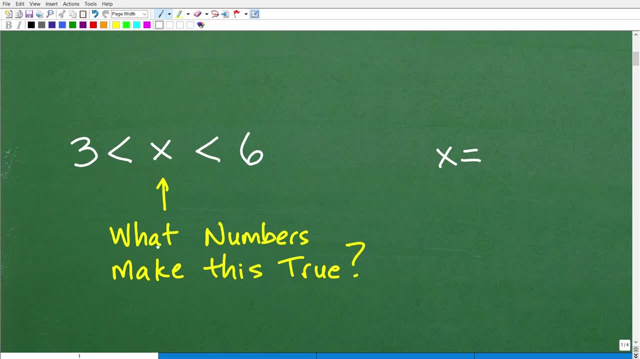 inequality. Well, basically, what number, numbers, number or numbers? let me kind of fix that for a second. make this true, This statement right here. true? Well then, that is a solution. So let's go ahead and start. 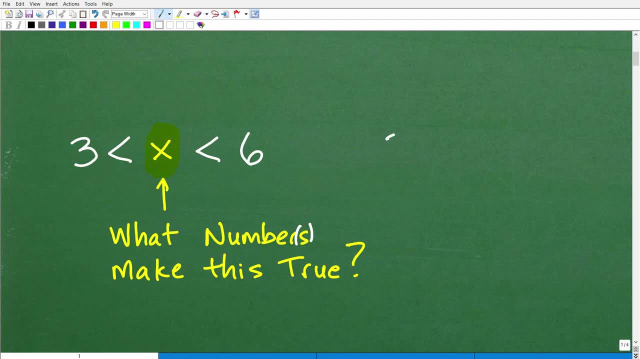 replacing x with some actual numbers. Let's plug in for, just to make this simple, let's plug in four And let's see if this makes sense. Okay, So is four greater than three? Yes, this checks right here. And at the same time, four is less than six. All right, so four is what we call a solution. 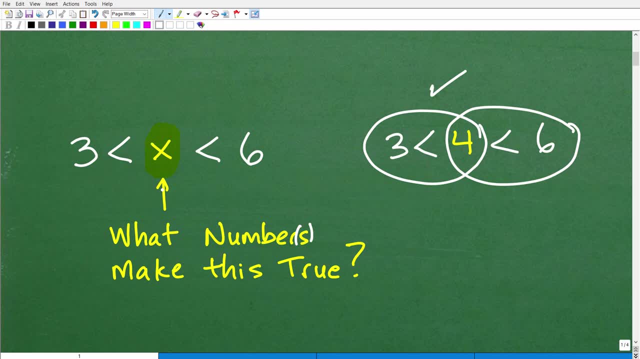 Okay, it is a solution to this inequality. Let me just kind of say that Now is it the only solution, So we could say: all right, four is a solution. Well, let's plug in another number. How about five? Okay, so let's take a look at if five works. Is five greater than three? Yes, Is five. 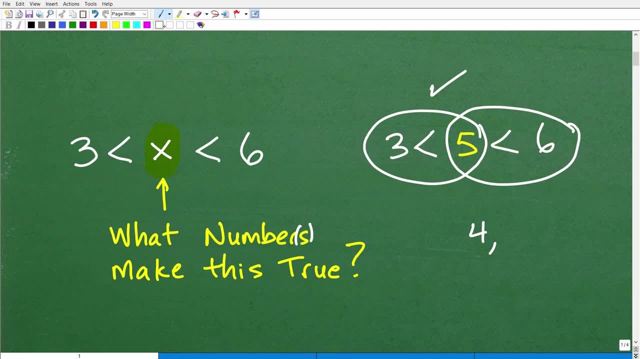 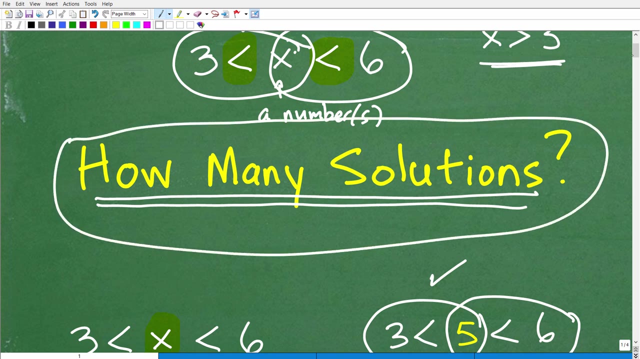 less than six as well. Yes, it is So. five works as well. Okay, so these are examples of solutions to this inequality, But again, I wanted to know right here how many solutions. That's the question, not give me a couple of solutions. So how many solutions do we have? Well, now, 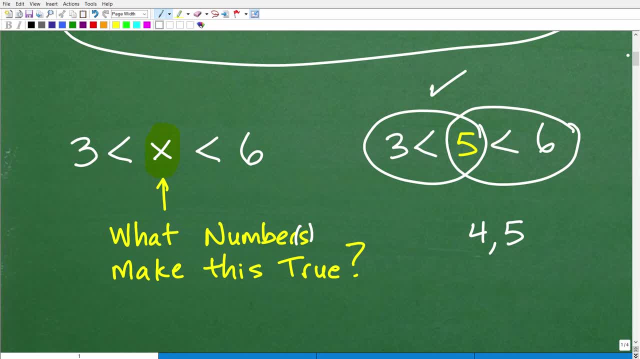 if you start looking at this, you're saying, well, hmm, well, can we just write a whole bunch more numbers? Let's say, how about 3.0001?? Okay, is that a solution? Well, is 3.001 greater than three? Yes, that is, That is true. Okay, and is 3.001 at the same time? 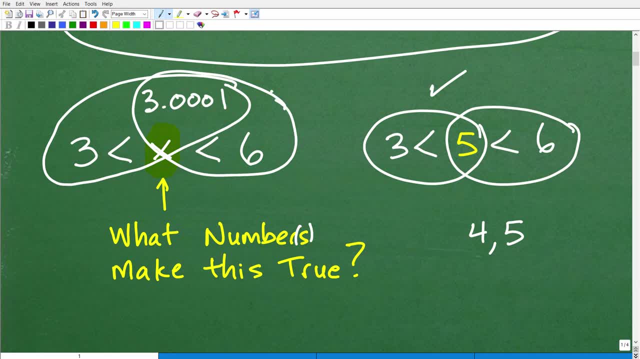 less than six. Yes, that's true as well. So hopefully this right here is going to give you a little bit of a kind of indication to be like man. there's probably a lot of numbers that will satisfy this inequality, And this is the exact case. Okay, when it comes to inequality. 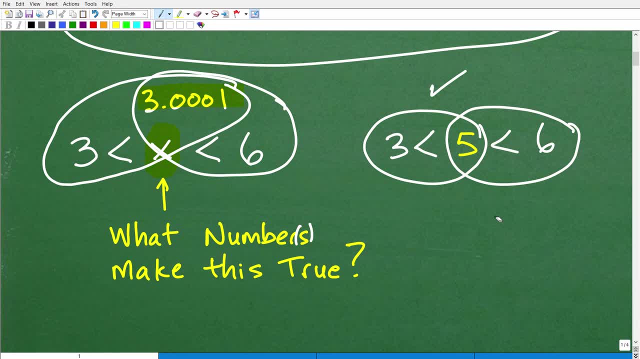 inequalities? there's never. it's not like algebra in terms of a basic equation like: 2x is equal to eight. Here, the solution to this equation is: x is equal to four. This has one solution, Okay, one and only one solution to this equation When it comes to inequalities. 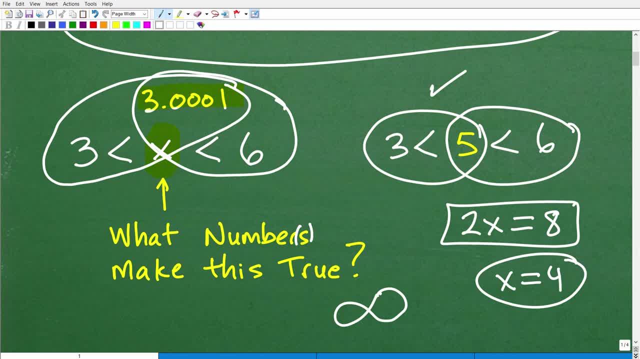 inequalities have infinite number of solutions. So if you put that down into the comment section, well, I must go ahead and give you a nice lovely little happy face and a plus plus 130% and multiple stars, because that is pretty awesome. Okay, inequalities have infinite amount. 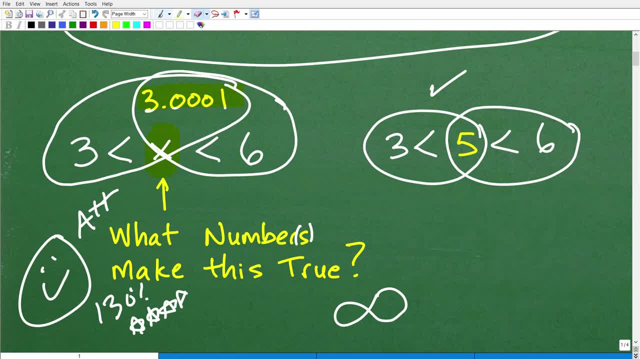 of solutions. Let's take a look at another basic example. How about x is greater than three? Okay, so here is a nice basic inequality. How many numbers satisfy this inequality? Okay, make this true. Well, any number that is greater than three makes this true. How many numbers are in fact? 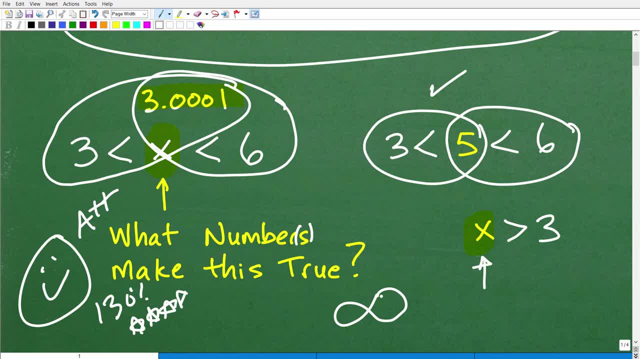 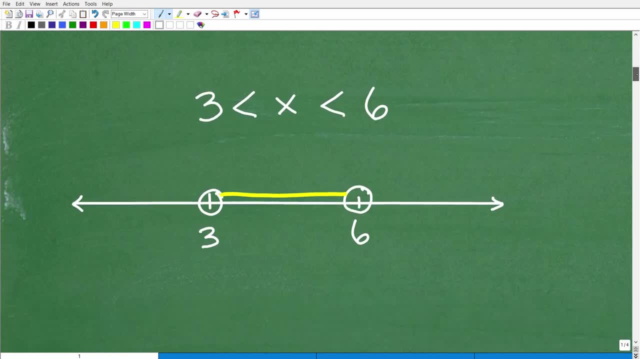 greater than three. Okay, so here is a nice basic inequality. How many numbers satisfy this inequality? Okay, this brings me to kind of like my main kind of point in this particular video here, this little micro lesson, is that inequalities, unlike equations, okay- are typically going to have. 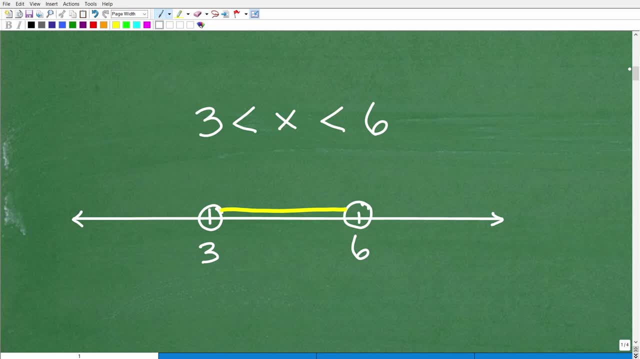 equations are going to have. generally speaking, I've got it because there's all sorts of type of equations in mathematics, But typically- for like most of you out there studying any sort of algebra course- are going to have a finite amount of solutions. So if you're going to have a finite 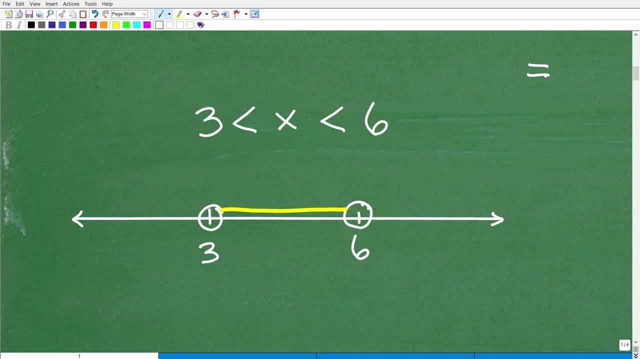 number of solutions. okay, so when you see things with equal signs, this is going to have a fixed number of solutions. inequalities always have an infinite number of solutions, So because of that, we want to express our answers with graphs. Okay, so that's why it's important to know how to graph. 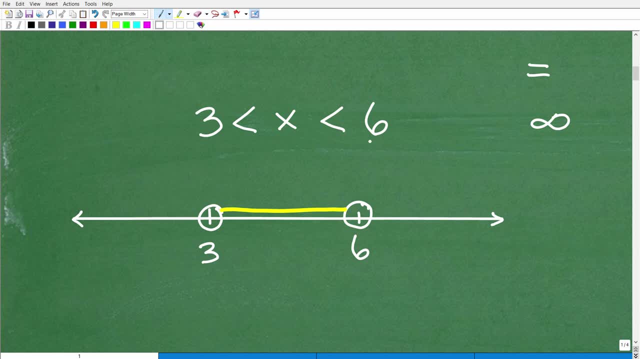 inequality. So let's go to take a look at the graph for this one. All right, So again, all numbers that are greater than three at the same time less than six. Well, let's plot three lines So we can kind of see that graphically these are going to be what we call open circles. 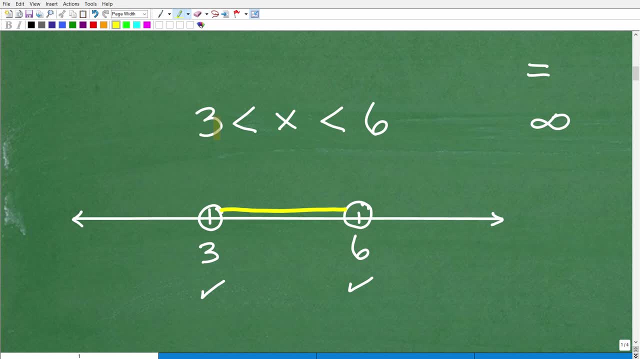 meaning that the solution to this inequality does not include this number. Okay, so for example, three, right here. three is not greater than three. Now, if I had is let's kind of fix this up right here. If this was our inequality, three is less than or equal to x is less than. is less than six. 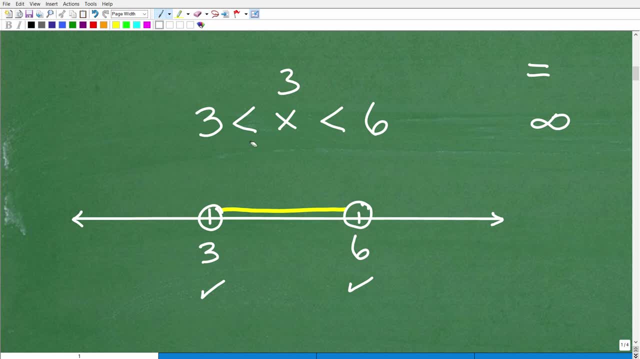 if I have three right here, then this would be less than or equal to three. So if I had three, satisfy this equation. but that's not the case. This is just a quick video on inequalities. If you're kind of confused about this, you might want to start off by checking out my more basic 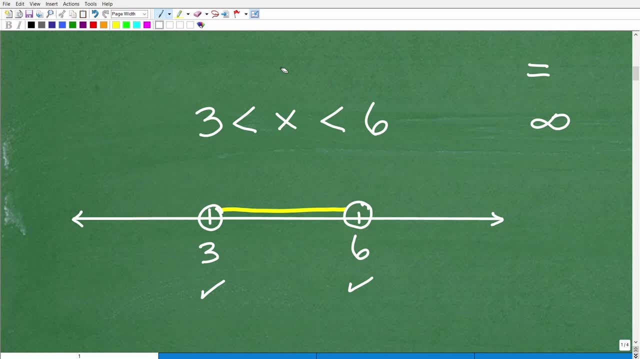 videos on inequalities or maybe check out one of my courses like pre algebra. I really kind of cover all this thoroughly. But let's just kind of get back to why we have graphs that go with inequalities, because graphs illustrate that, hey, we're talking about an. 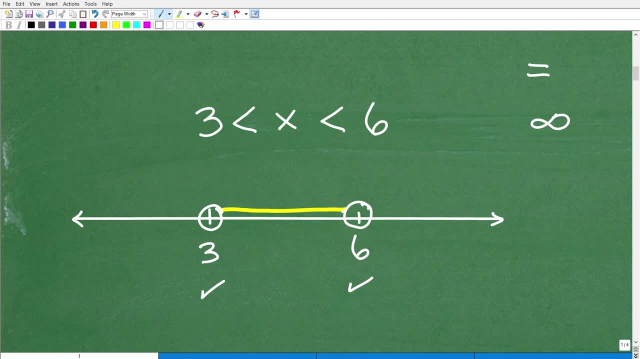 infinite amount of points. So, anyways, to get back here, to graph this particular inequality, we're going to have to do a little bit of math. So we're going to have to do a little bit of math to get back to this particular inequality. all the numbers- okay x- that are greater than 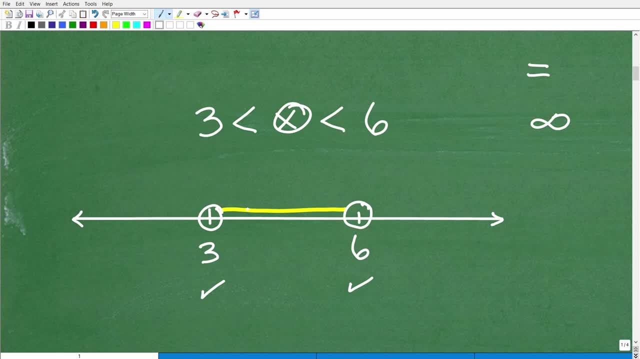 three, but the same time, less than six, fall between this range right here. Okay, so greater than three and less than six are all these numbers. So this is the way you would graph. the solution to this inequality is we plot this- numbers three and six- and then we draw a line. 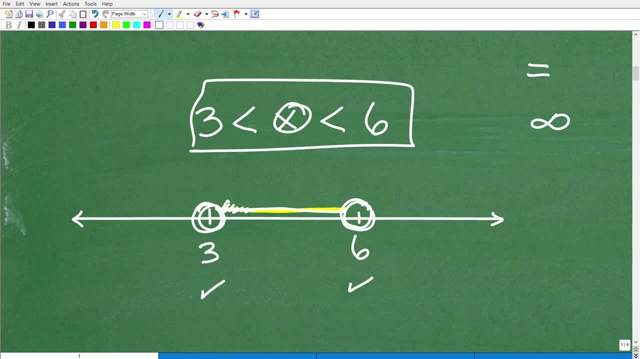 right there, And these are open circles. okay, right, like so. So I will kind of just make this nice and clear: if we have equal to you would fill in these circles like like so. but just you know, asking yourself how many numbers are between three and six. 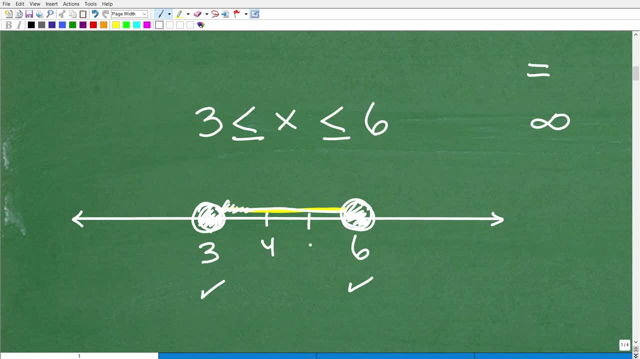 well, you know, it's not just like, oh, there's four and there's five, there's like two numbers, no, there's all the decimal values between these two numbers is an infinite amount of numbers between here and here. okay, so you might not think that, but that's in fact the case. so again, the really the big point to